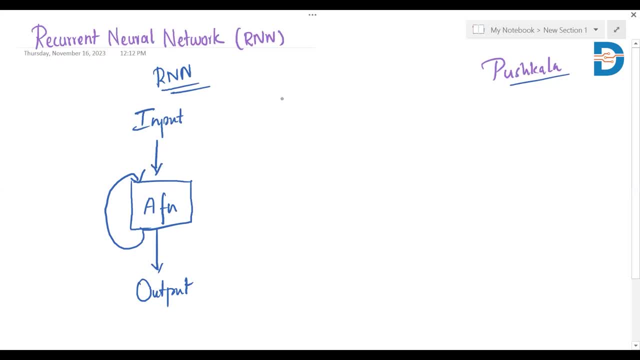 So let's say you have to give a sequence of inputs To predict the next output. So sequence in the sense let's say I have 10 inputs and I'll have to predict next single output. So in this case in most of the neural networks the number of inputs is fixed up. 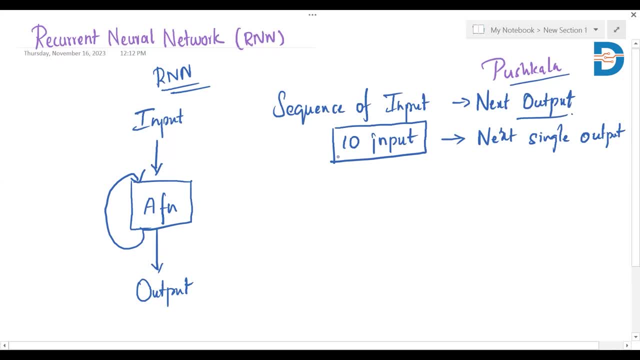 If it is 10 inputs. each time the user comes up have to give 10 inputs and single output will be given by the neural network. This is general in most of the neural networks, Whereas in recurrent neural networks you can give any number of inputs, It's not specified the sequence have to be of a particular length You can. 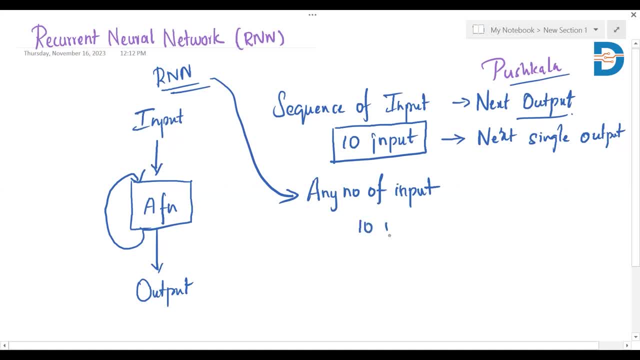 give any number of inputs. I can give 10 inputs and ask for next single output. or I can give 4 inputs and ask for next output. I can do any of the input sequence. Input sequence doesn't have a proper size. It can be of changing sizes. That is why RNN architecture is different. 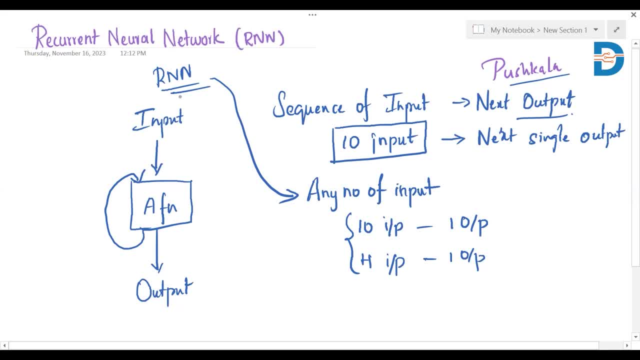 from others When you have to handle the inputs with sequences of different lengths. you can give any number of inputs. I can give 10 inputs and ask for next single output. Or I can give 4 inputs and ask for next output. I can do any of the. 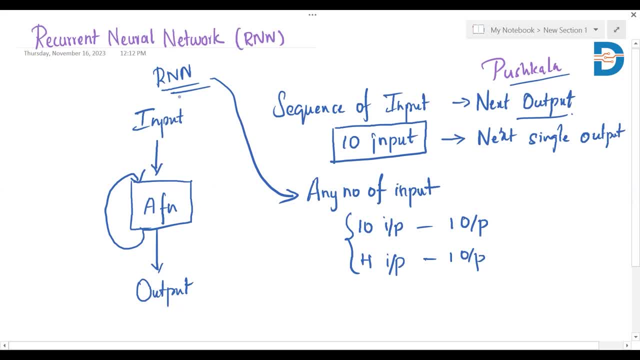 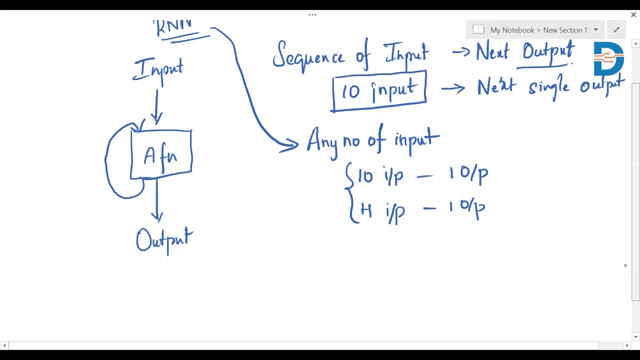 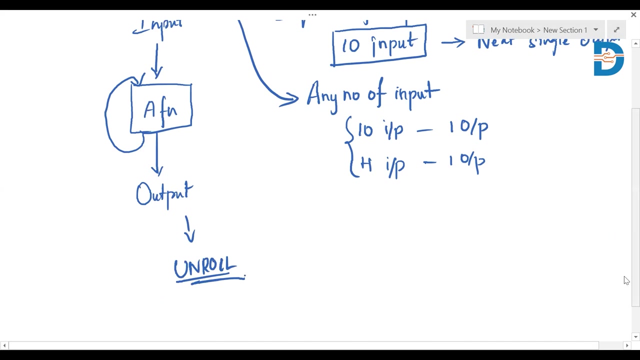 inputs That are different from one another. you can go for RNN, And how does RNN architecture work? It just has the extra feedback loop. And how does it differ from the other networks? So let's say you have, let's unroll this, Let us unroll this neural network, Just yes. 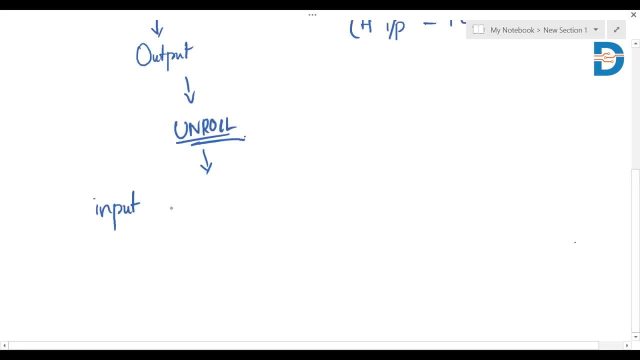 I have 3 inputs. Let's say this is input 1. And I'll be giving that to the first activation function, Isn't it? And it will give me the output 1.. This is usual, But in recurrent neural network I need to give the input 2.. In that case I'll have a summation here And then I'll.